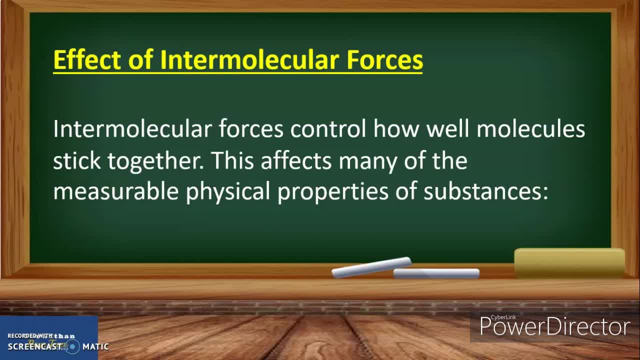 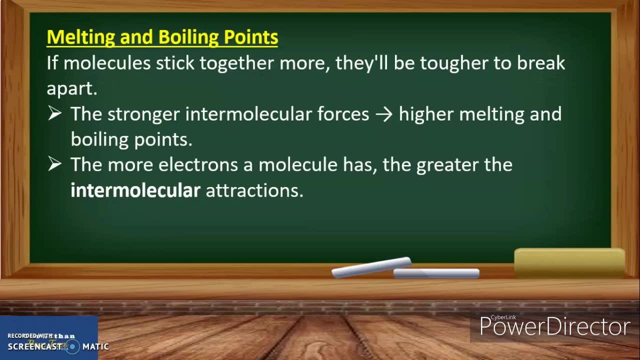 intermolecular forces control how well molecules stick together. this affects many of the measurable physical properties of substances. let's have melting and boiling points. if molecules stick together more, they'll be tougher to break apart. so let's have the properties: the stronger intermolecular forces, the higher melting and 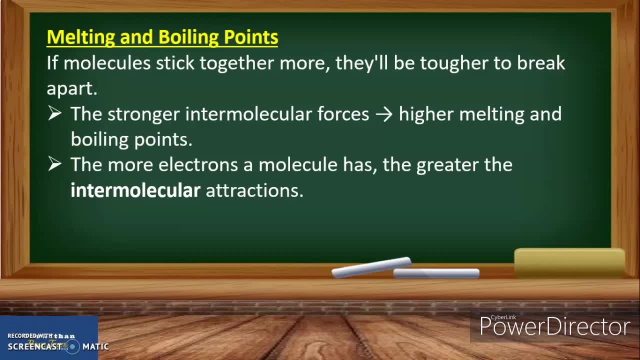 boiling points. so it's a good point. so if the intermolecular forces is higher or strong, so you will observe that the melting and the boiling point is also high. so this is the reason why if the liquid is thicker or viscous, the melting point is higher. 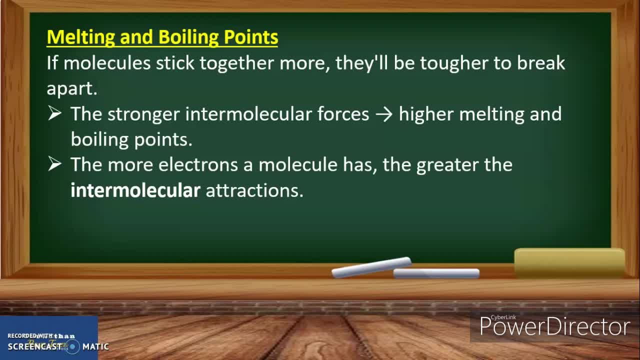 and the boiling point also is higher. if the liquid has a very low intermolecular force, like that of, example, of London forces, okay. or for the dipole dipole, a dipole type of liquid, the melting point and the boiling point is low, so the more electrons a 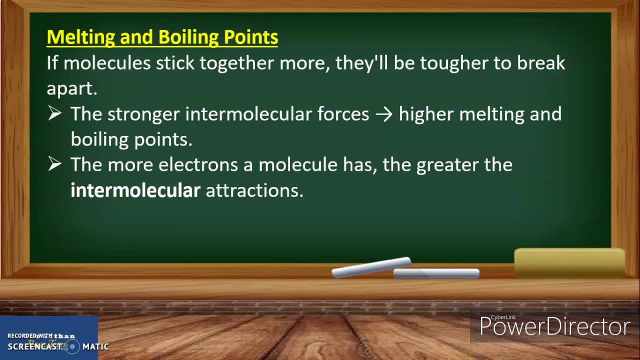 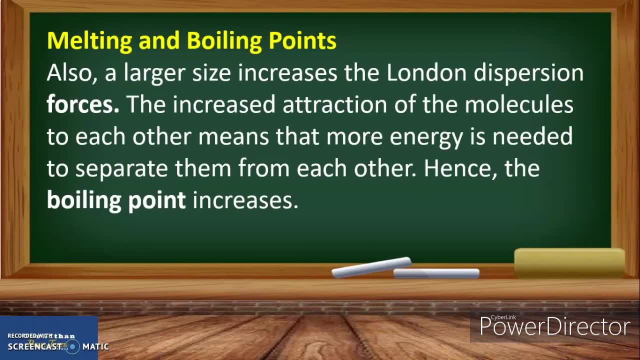 molecule has, the greater intermolecular attractions. also, a larger size increases the London dispersion forces. the increased attraction of the molecules to each other means that more is needed to separate them from each other. hence the boiling point increases. so same through with other things. okay so if they are huge or large, okay so the 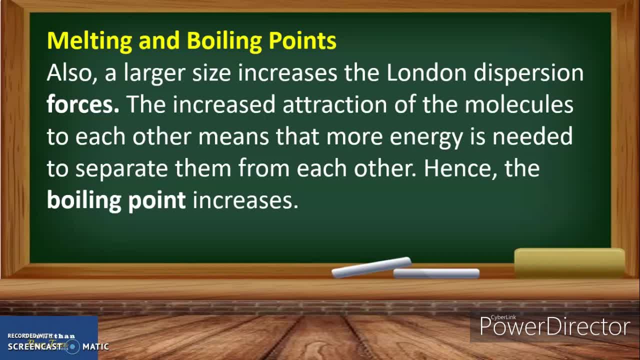 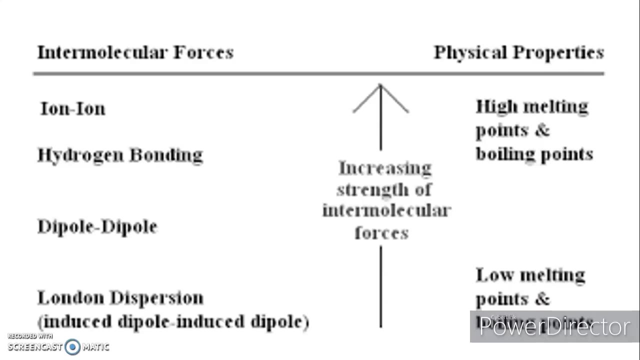 intermolecular forces also increases, so the more you need energy- for example, you are going to hit something, so you need heat energy for that one in order to separate this intermolecular forces- and hence the boiling point increases. so let's take a closer look of the summary of this boiling and melting points when. 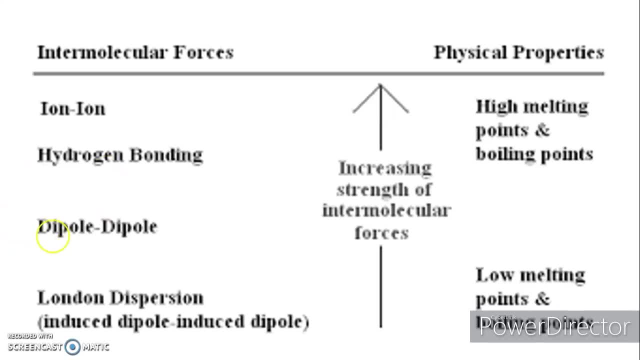 it comes to the intermolecular forces. okay, so, as you can see on the left hand portion, these are the inter or the types of the intermolecular forces. so we have the London dispersion, dipole-dipole, hydrogen bonding and ion-ion, or we can include also the 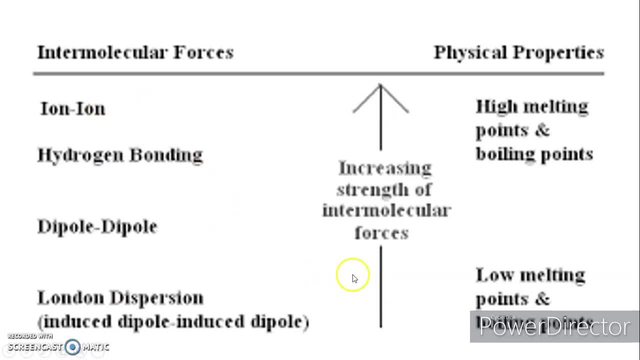 ion-dipole type. so the strength of intermolecular forces increases. okay, as the type of intermolecular forces okay is concerned, then the physical properties like the melting and boiling point also increases. that is why we observe that in hydrogen bonding like water, okay the boiling point. 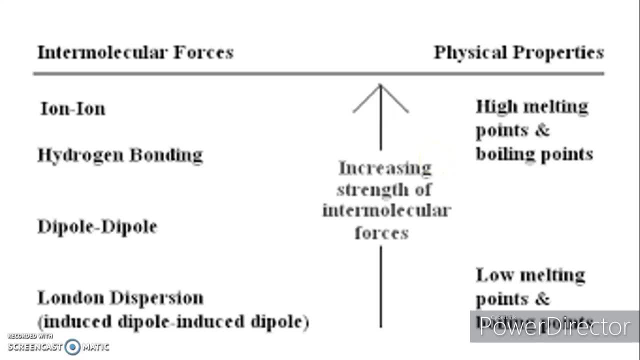 is higher. so the boiling point in lower altitude is 100 degree Celsius. for higher altitude the boiling point vary. then we have the ion-ion or ion-dipole, okay, so the boiling point also includes the boiling point as well. so if you put something on water like sugar or salt, okay, or other things, the 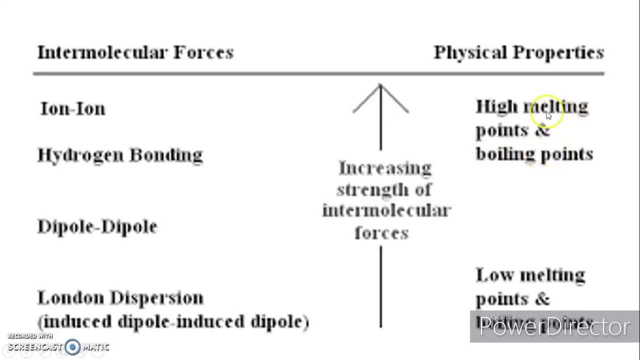 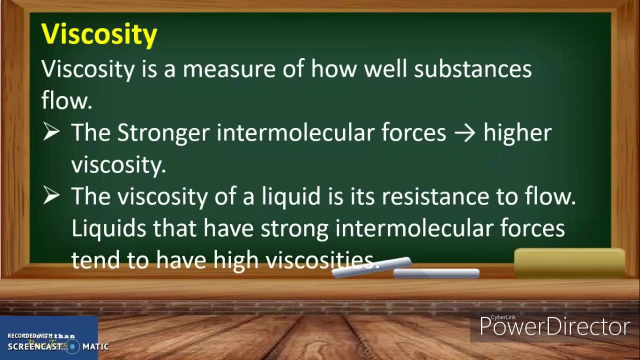 boiling point will also increase same through with the melting points: viscosity. viscosity is a measure of how well substances flow. the stronger intermolecular forces, the higher viscosity. the viscosity of a liquid is its resistance to flow. liquids that have strong intermolecular forces tend to have high viscosity, like, for example, we have gasoline and we have diesel. okay, so 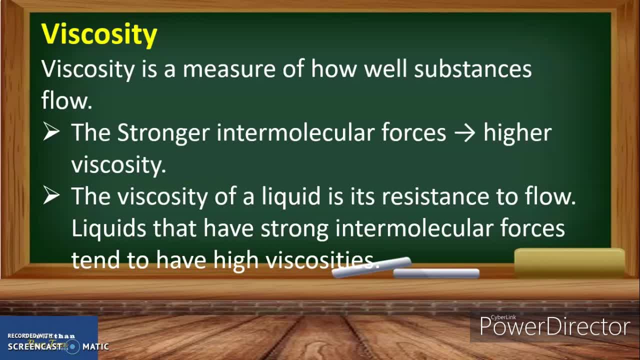 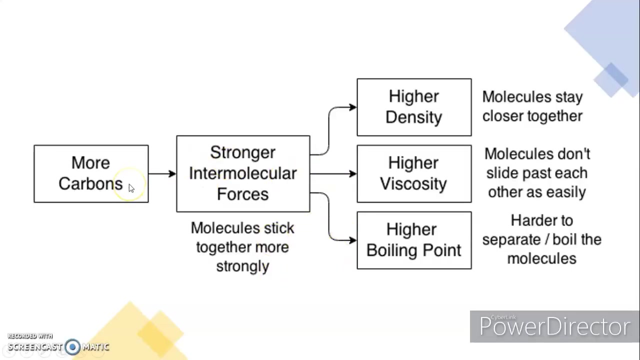 the other one is more viscous. the other one is less viscous. gasoline flow is easily compared to diesel. this is due to the intermolecular forces present in the two types of liquids. so diesel has a strong or heavy- strong intermolecular forces, while gasoline have weak intermolecular forces. so that example. 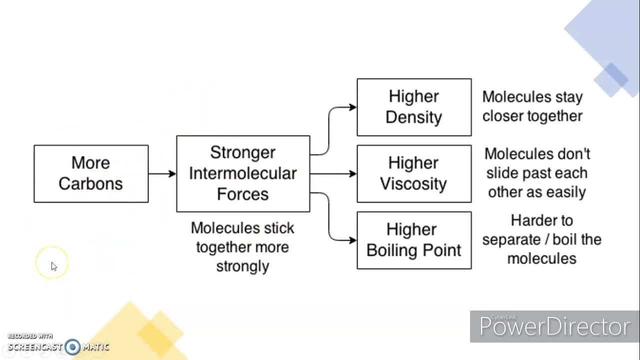 pertains to this illustration. diesel has a long chain of carbon compared to gasoline, so you observe stronger intermolecular forces. some molecules stick together more strongly. you will observe higher density, higher viscosity and higher boiling point. some molecules stay closer together. molecules don't slide fast between other as easily. harder to separate boil the. 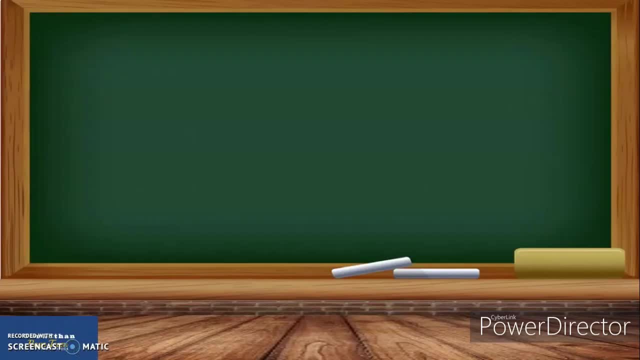 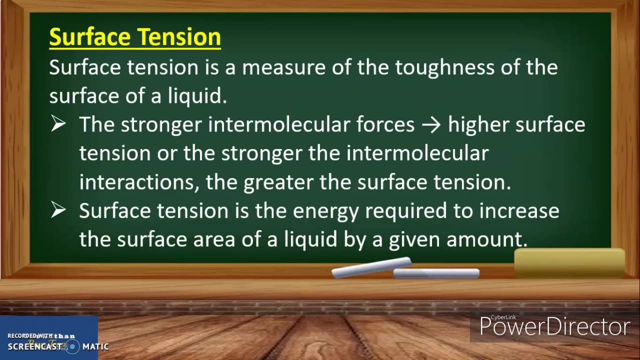 molecules surface tension. surface tension is a measure of the toughness of the surface of a liquid. the stronger intermolecular forces, the higher surface tension, or the stronger intermolecular interactions, the greater the surface tension. surface tension is the energy required to increase the surface area of a liquid by a given amount. 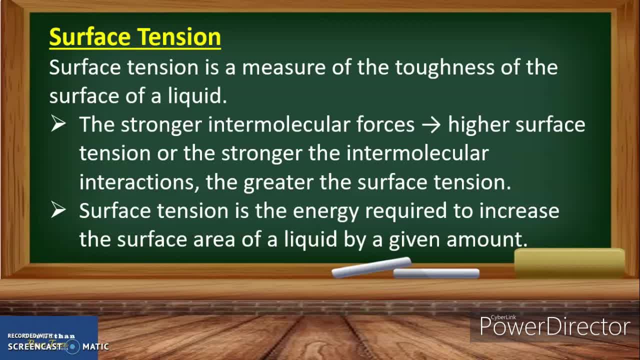 so if you're going to compare condensed milk with water, okay, condensed milk has a higher surface tension compared to water, so you can place heavier objects or objects with high density in condensed milk without sinking, while in water, when you put something high density, it will sink easily. so that is a good analogy to imagine surface tension between condensed milk and. 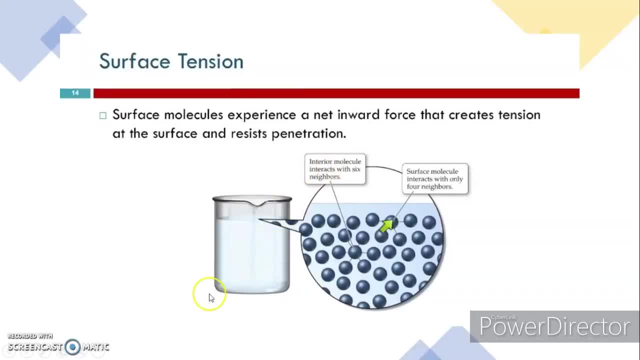 water surface molecules experience a net inward force that creates tension at the surface between condensed milk and water surface molecules experience a net inward force that creates tension at the surface and this is penetration. so that is the very good example of condensed milk. the interior molecule interacts with six neighbors there it's like a network or a web service molecule interacts with. 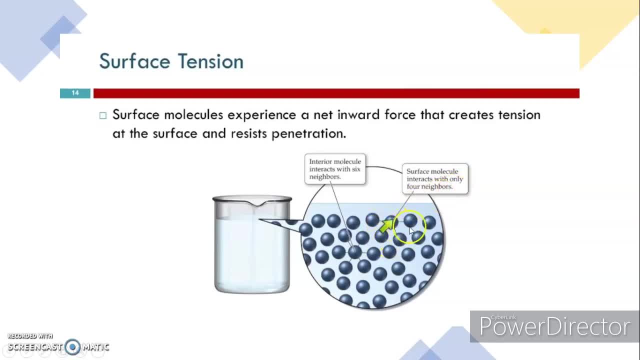 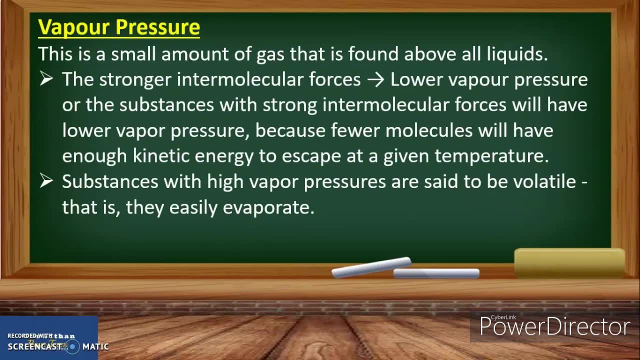 only four neighbors their vapor pressure. this is a small amount of gas that is found above all liquids and it is a very good example of condensed milk. and it is a very good example of condensed milk. the stronger intermolecular forces is the lower vapor pressure, or the substances with the strong. 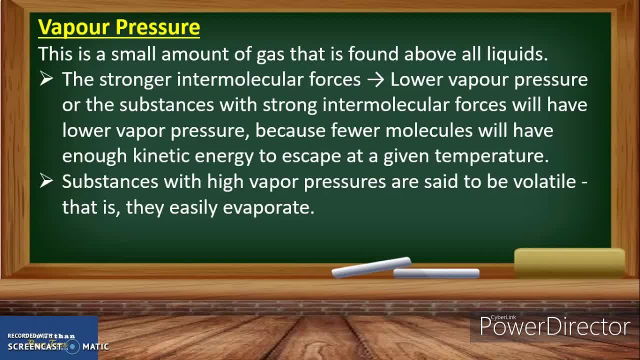 intermolecular forces will have lower vapor pressure because power molecules will have enough kinetic energy to escape at a given temperature. substances with high vapor pressure are said to be volatile, that is, they easily evaporate. so when there is a lead on the content of condensed milk, 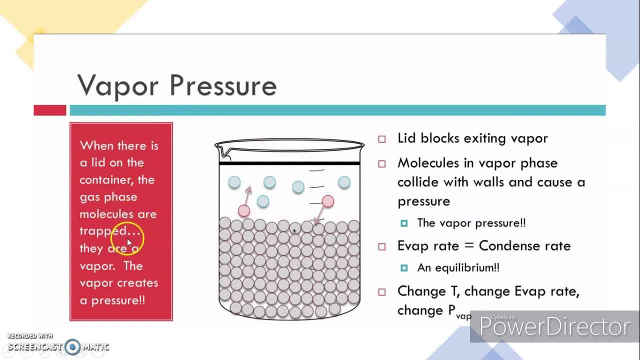 container the gas-based molecules are trapped. they are a vapor, so the vapor creates a pressure. that's why we call them vapor pressure. lead blocks exiting vapor molecules in a vapor phase collide with walls and cause a pressure, so that is called vapor pressure. so the evaporated rate is equal to the condensed rate. that is an equilibrium. 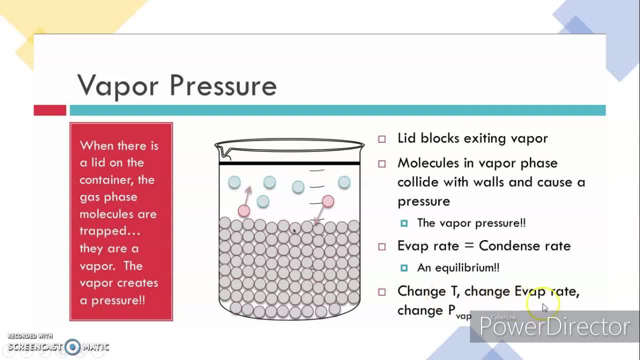 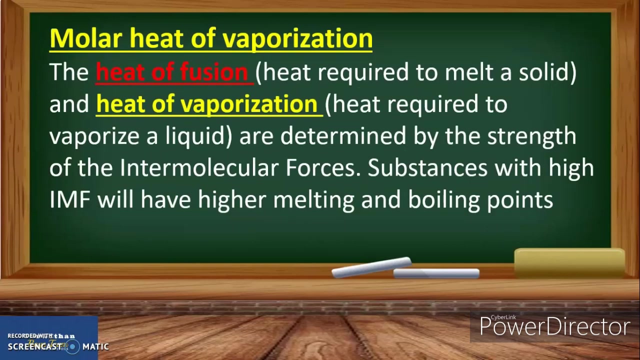 So change in temperature, change in evaporation rate and change in vapor pressure. So when you boil something, when you cover the lid or you put the lid, it will also create pressure. So that is called vapor pressure from the steam of the water. Okay, Molar heat of vaporization. So the heat of fusion and the heat of vaporization. So what is the difference between the two? 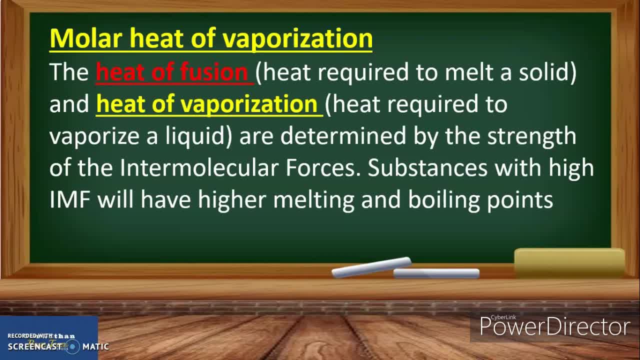 When we say the heat of fusion, this is the heat required to melt a solid, While heat of vaporization is the heat required to vaporize a liquid. So these are determined by the strength of the vaporization, The strength of the intermolecular forces. Substances with high intermolecular forces will have higher melting and boiling points. 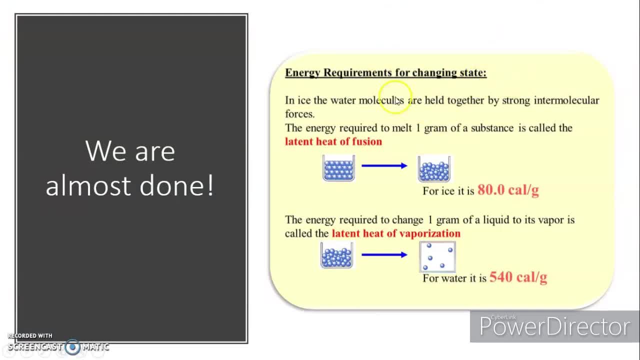 So energy requirements for changing the state. In ice the water molecules are held together by strong intermolecular forces. The energy required to melt one gram of a substance is called the latent heat of fusion. So take note from solid to liquid. For ice it requires 80 calories per gram.